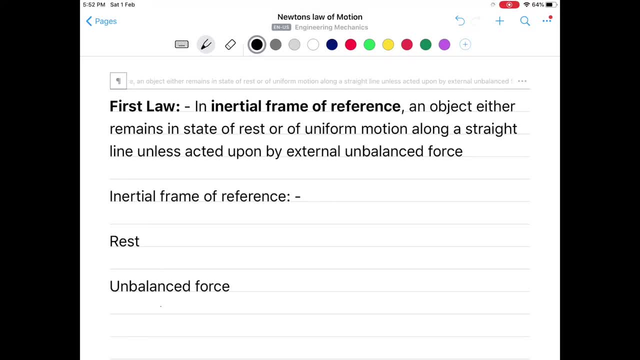 Inertial frame of reference means if a viewer who is just seeing that motion, if his velocity is constant, right. So inertial frame of reference means velocity of viewer is constant, It can be zero or it can be moving with a constant velocity, but it should not accelerate, right? So this is very important. So this is inertial frame of reference. Second thing is when there is no 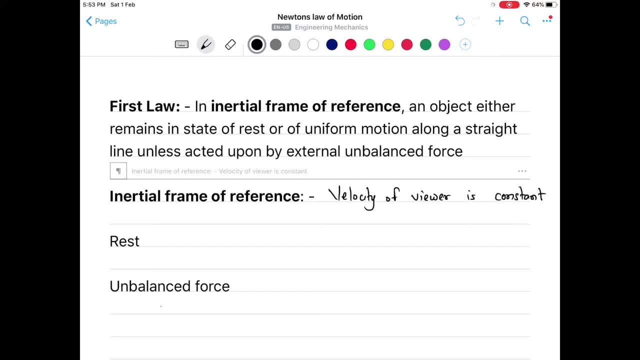 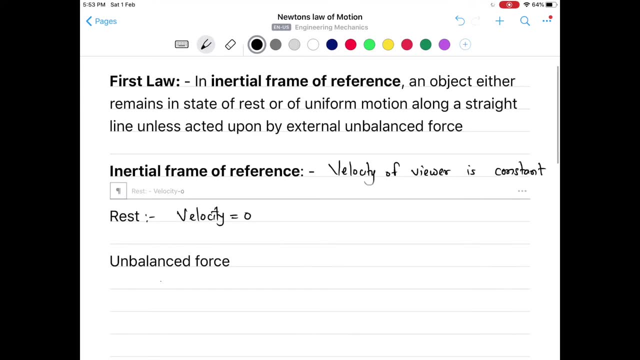 force acting on it, then the object remains in a state of rest. So what do you mean by state of rest? Rest means velocity equal to zero right. And the third thing that you have to remember is uniform motion along a straight line. Uniform motion means- I'll just write- uniform motion. that means velocity is constant. 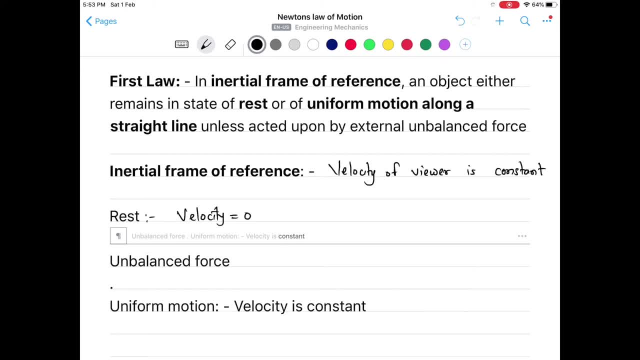 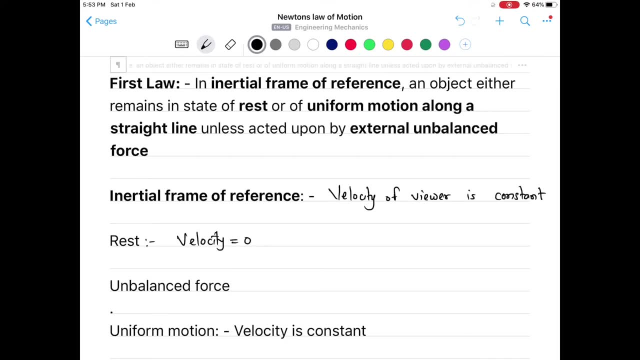 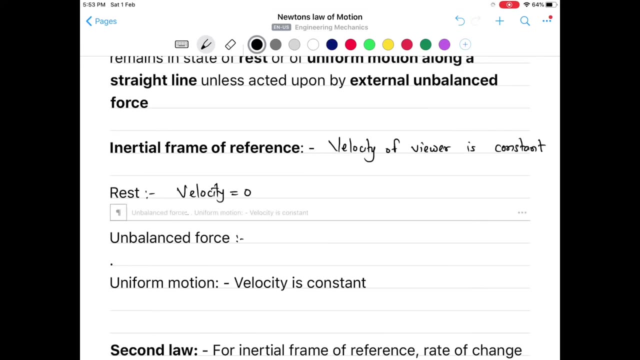 So uniform motion on a straight line. and the fourth thing is external unbalanced force, right? So you have to remember that whenever there is no external unbalanced force, So what do you mean by external unbalanced force? is net force equal to zero? 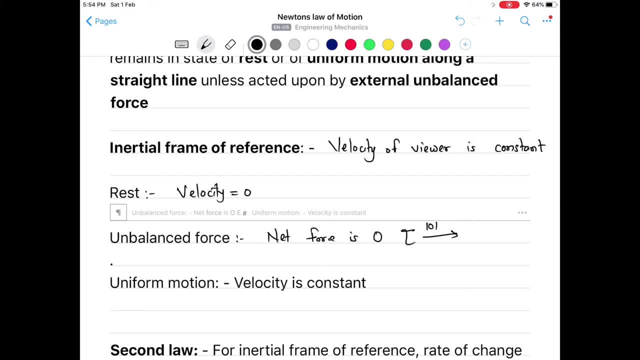 So there can be a force of ten new in this direction and in equal and opposite force of 10 newton in this direction. so that means this force cancel, cancels out each other, right, that means the net force is zero. so this is a meaning of unbalanced force. that means net force equal to zero, so there can be force acting on it. 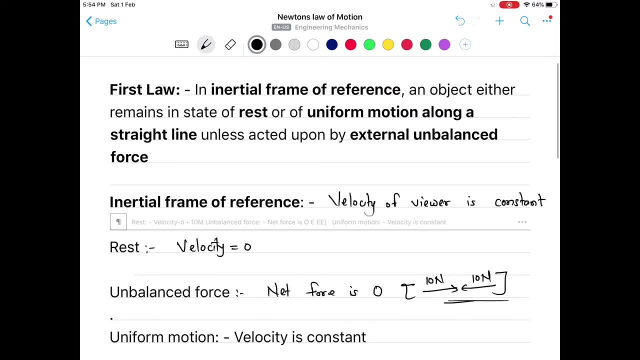 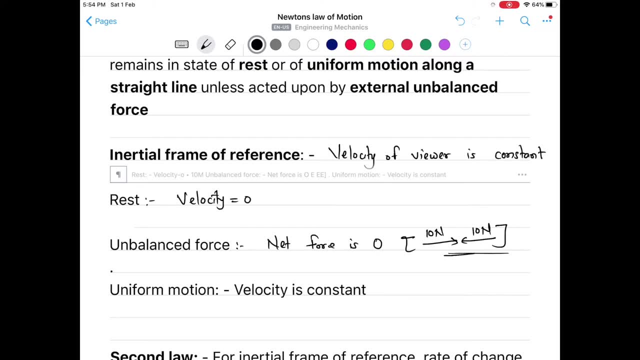 but the resultant of that force, or the net force, has to be zero. so what does it mean? i will just tell you once again in simple words. so if there is no net force acting on the body, no net force means there is no unbalanced external force. force can be internal. internal forces are mostly. 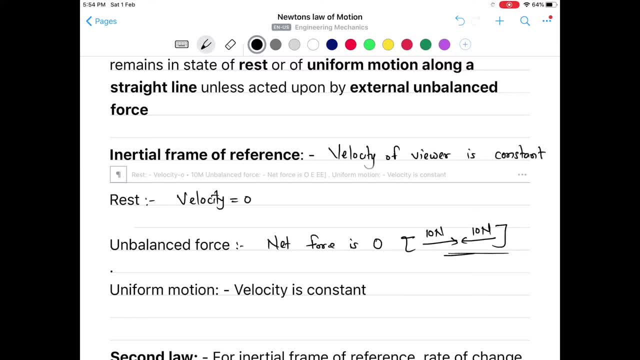 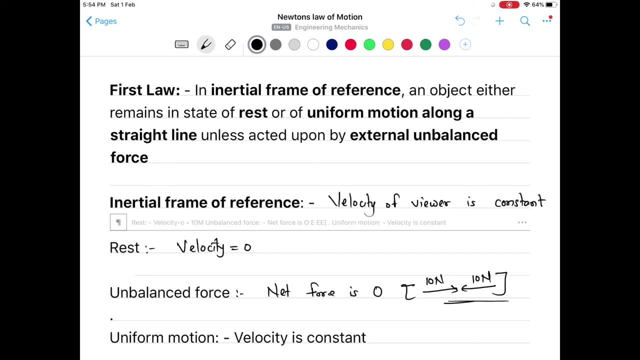 balanced force. so there has to be an external force which has to be unbalanced, right? so if there is no external unbalanced force, then in the inertial frame of reference the body will remain in a state of rest or of uniform motion. that means the body, body's velocity will remain. 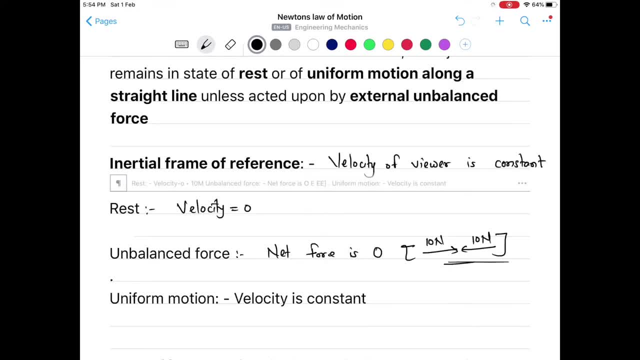 constant and that if that body is moving, then that body will continue to move along a straight line. it doesn't have to move along along a circular path. if it is moving, then there is some kind of force acting on it to keep that body. there is motion in along a circular path, right? so you have to remember this thing. 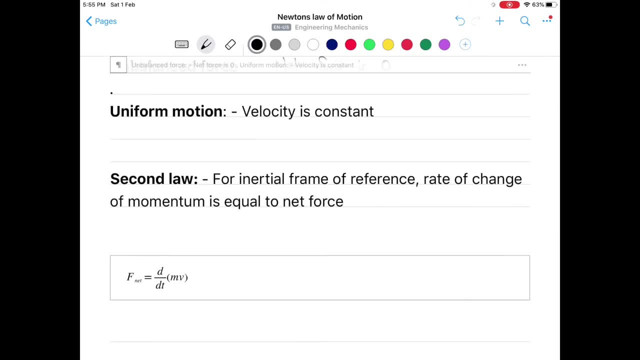 now let us move to the second, second law of motion. it says that in inertial frame of reference, the rate of change of momentum is equal to the net force right. the first law was stating that when there was no net force acting on the body, what will be the state of motion of a body? 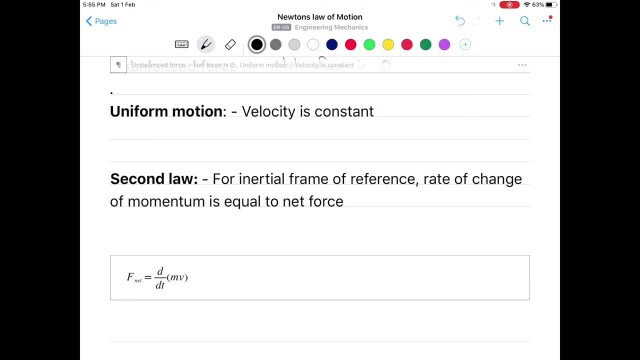 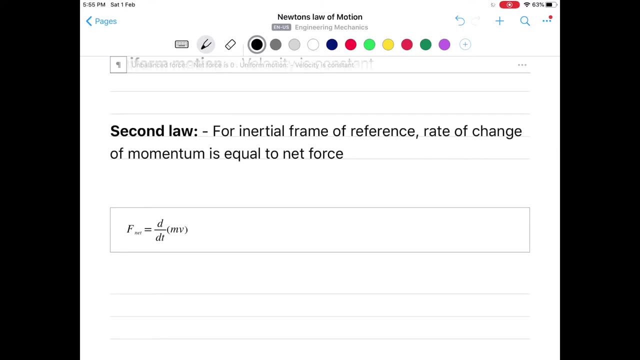 now second law state goes ahead and state that suppose if there is a force acting on the body, then how the body's motion will change. right, so here it says: newton law says that if there is a net force, that is f net, acting on the body, then the rate of change 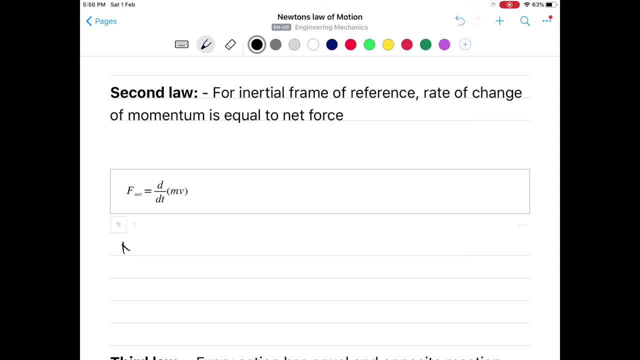 of momentum. momentum is mass into velocity and just write: momentum is equal to mass into velocity. so it says that force is equal to rate of change of momentum. right, many of the places it is stated that force equal to mass into acceleration, but that is true only in some particular cases. 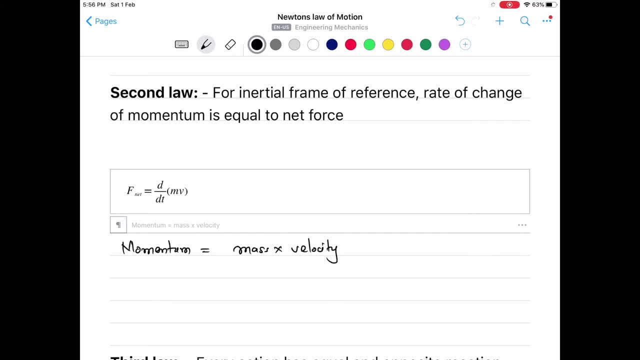 and in engine mechanics it is mostly true- force equal to mass into acceleration. but there is a step in between right. so what we can do is we can write this derivative and we can split this right. that is, mass into dv by dt plus v into dm by dt. the first thing is mass into acceleration. 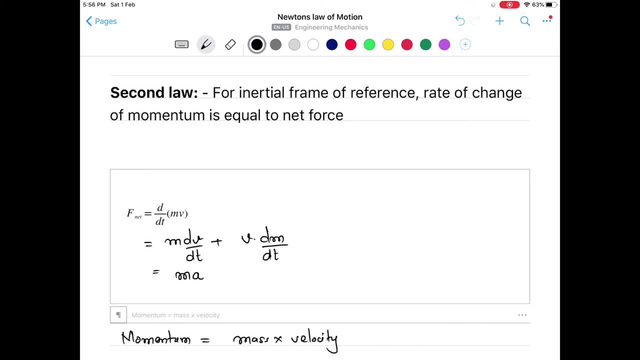 that is, change in rate of change of velocity with respect to time is acceleration. so this term has an acceleration and second term. in most of the cases in engineering mechanics, or in most of the general application, this, for the second term, becomes zero. right, there is no change in mass. 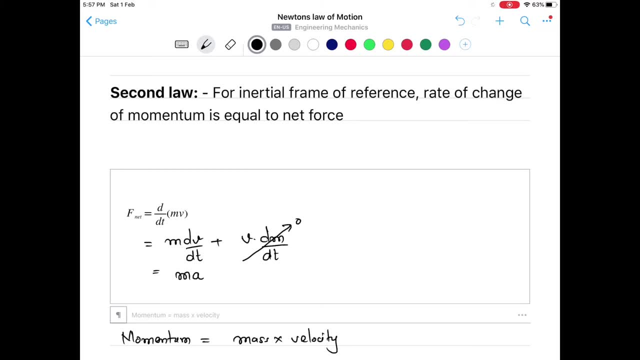 so there is an example for changing. my suppose. if you have, if there is a rocket right and if you have just ignited it, so the mass of the rocket will will gradually decrease. so at that place, when your object of study is rocket, you cannot ignore the second term, that is, rate of change. 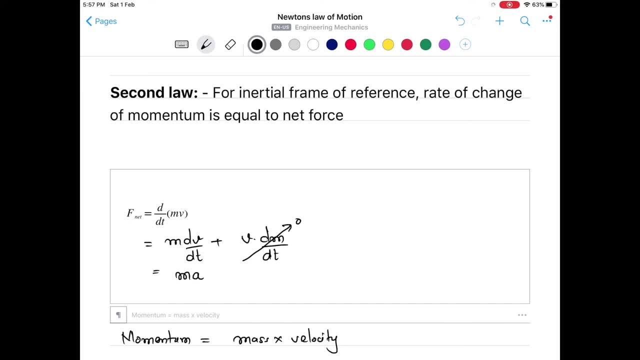 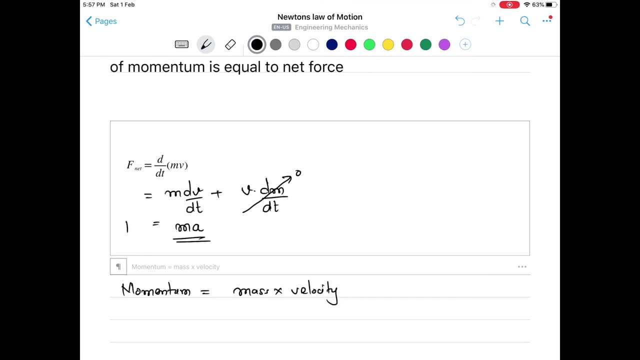 of mass, but almost all the problems in engineering mechanics. mass will remain constant, but you have to be careful with this. so this is the second law of motion, that is, force equal to mass into acceleration. but you have to remember at the back of your mind that it is not mass interaction, it is 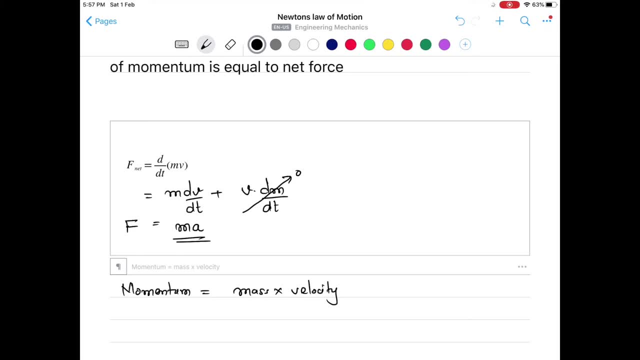 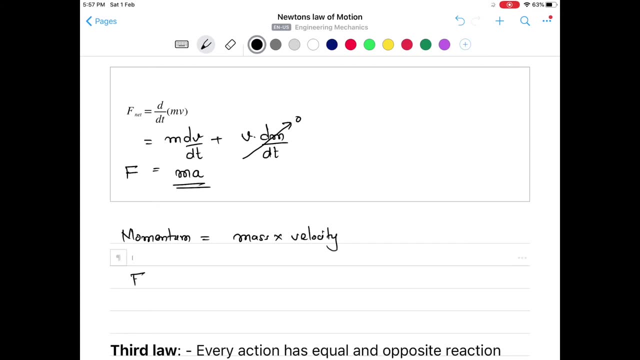 the rate of change of momentum. so whenever you write this force as the rate of change of momentum, you will never make a mistake. and here you have to remember one more thing: that force, velocity and acceleration, all are vectors, right. that means it has magnitude and direction, right. so what does it mean? is see, mass is a scalar right, so force, 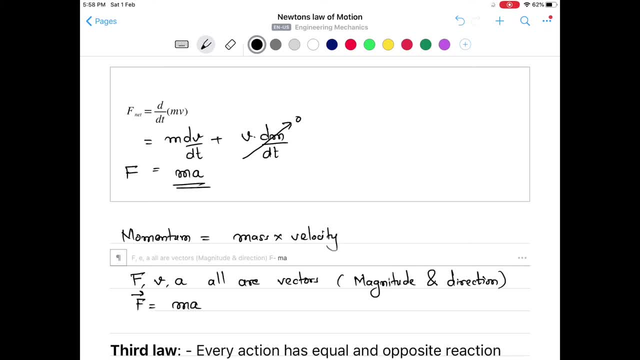 is equal to, let us say, mass into acceleration. force is a vector, so vector is bounded by a arrow above it and acceleration is also a vector. so what does it mean? that this term again is a vector and that it is equal to force. so the direction of force is equal to the direction of acceleration. 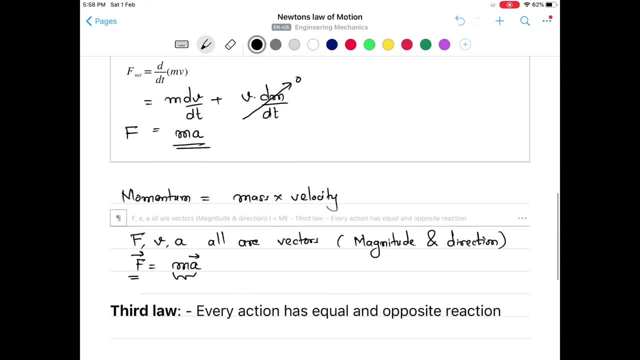 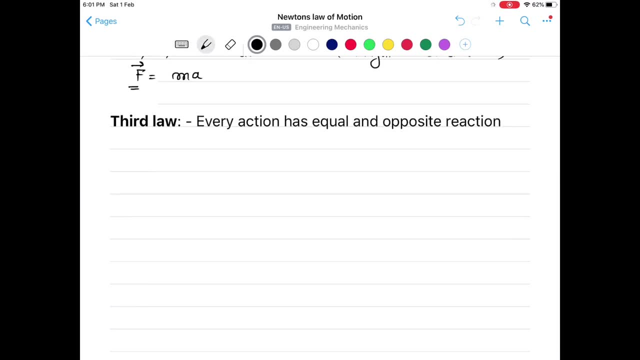 right. so we have to match the direction as well as in magnitude. so that thing you have to remember, or it has to be clear now. this is newton. third law of motion is very simple. it says that every action has equal and opposite direction. let us say that we are trying to push a wall away from 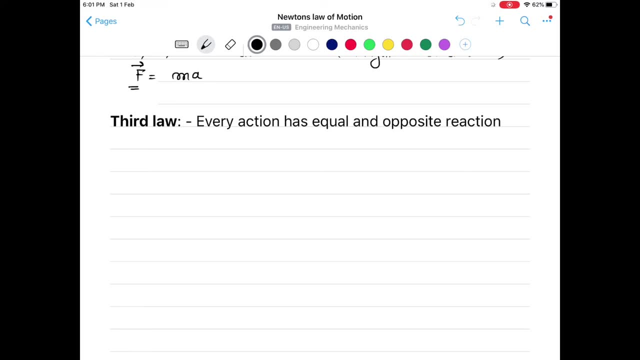 us right. so suppose a person is trying to push a wall, so that's why he's exerting some force f right person. I will just write a math that is force by person, right? So whenever the person is trying to push a wall apart, then the wall is again trying to resist it by an equal and 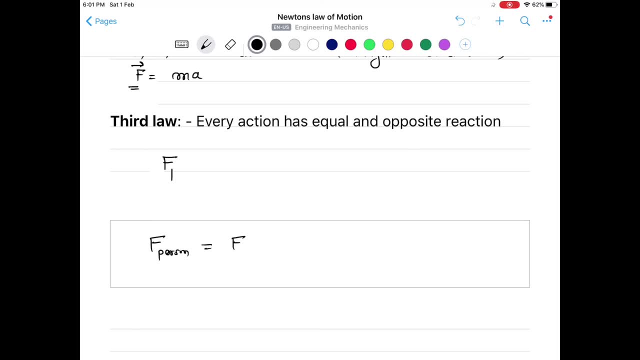 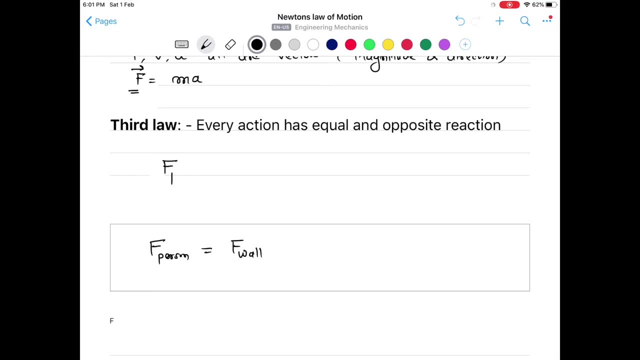 opposite force, So that force is also equal, but opposite F wall right, And that force will be equal and opposite right. So force on the wall will be opposite in direction but equal in magnitude. So that thing you have to remember. So that's all in this Newton. 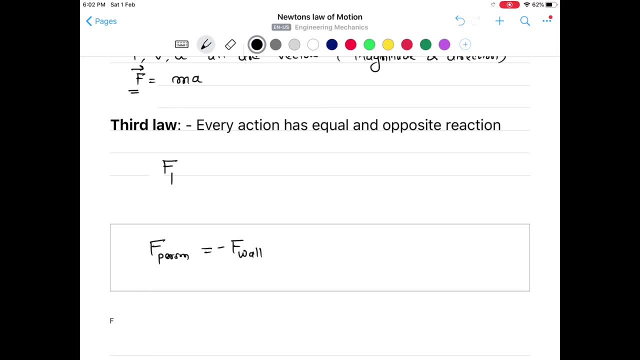 laws of motion. In the next video, we are going to study some of the basic mathematics that is applicable for vectors, because mostly we will be dealing with force, acceleration, velocity. All these things are vectors, right? So then, how to add it, how to subtract it?